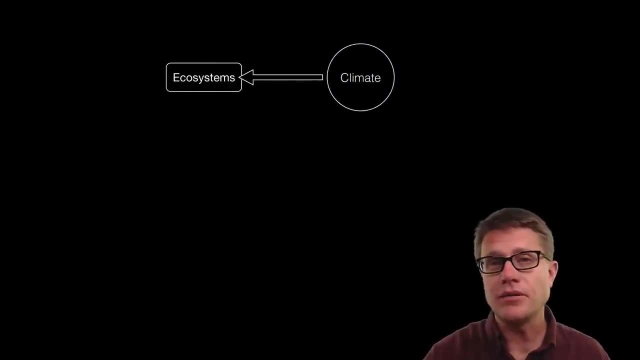 and that has affected ecosystems on our planet. But what is affecting the climate? It is where the earth is in relation to the sun, And so, as we have had changes in solar output, that is affecting the climate, And so, as we have had changes in solar output, that is affecting 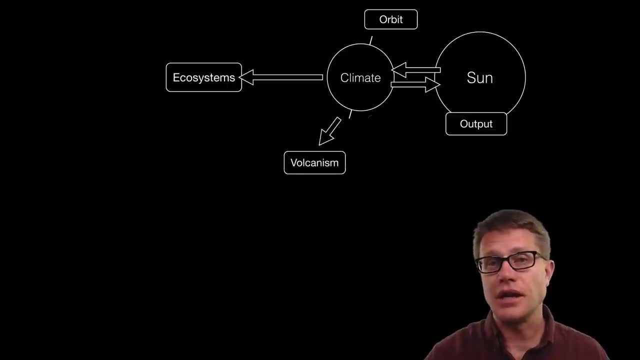 the climate, And so, as we have had changes in solar output, that is affecting the climate, As we have had slight changes in our orbit, or volcanoes, or plate tectonics, all of those things have affected our climate and therefore are affecting the ecosystems, Not only the. 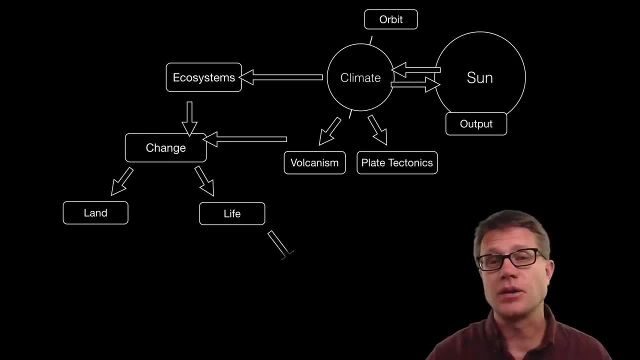 life, but also the land. At the worst level, it can cause what are called mass extinctions on our planet, where a number of species simply go away. Lots of times that is followed by adaptive radiation where different species come back, But for the most part, what happens? 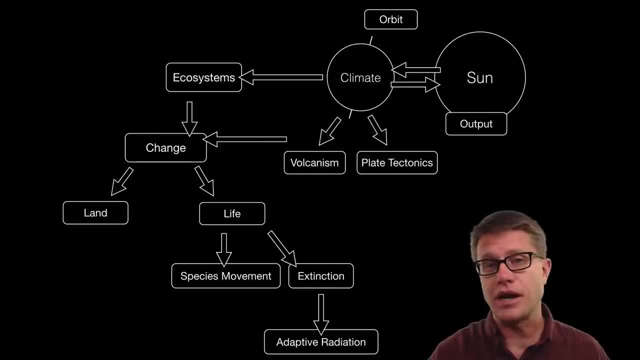 is, species have to respond, So species will move back and forth. So species will move back and forth as the climate changes. Now it also affects the abiotic factors, So the land on our planet, And so what happens after the land is destroyed or changed, is we have? 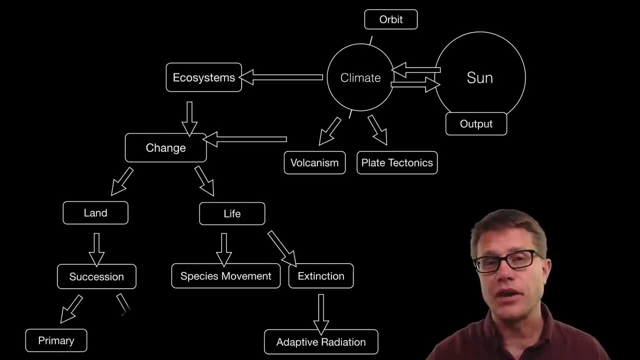 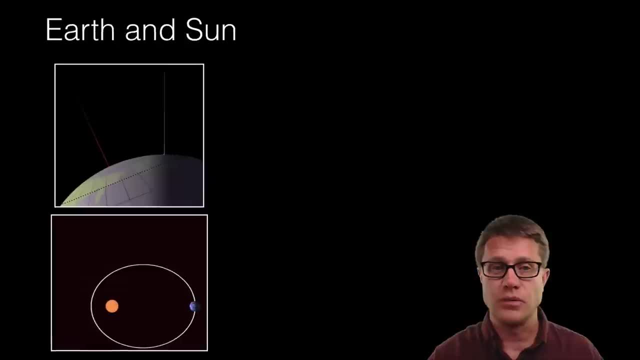 succession. as life moves back into that area, It can be either primary or secondary. In primary succession, the soil in the community is gone. In secondary, the soil in the community actually remains, And so what is affecting our climate is where the earth is in relation. 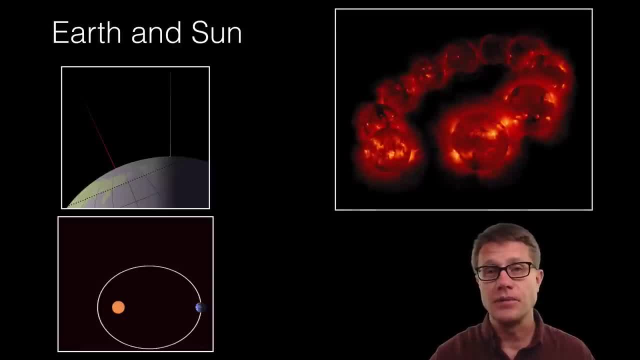 to the sun And scientists have noted that the sun changes over time. So we have these sunspots- 11 year sunspot cycles- but we have these larger changes in the output of the sun over thousands of years. We also find precession in the earth. As it spins, it also starts to. 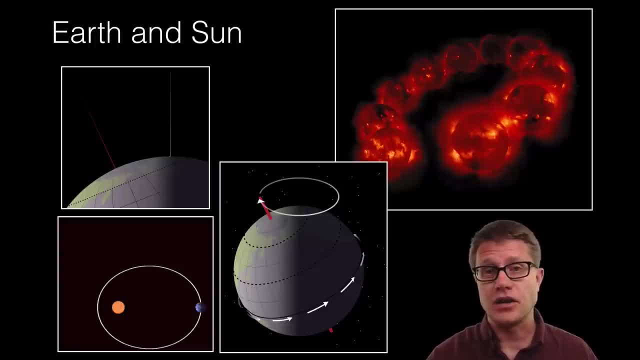 wobble over thousands of years And that causes changes in our climate. The pole starts to point in different directions, so we get varying amounts of light, And then we are also finding that there is precession in the orbit itself As it moves around over thousands of years. 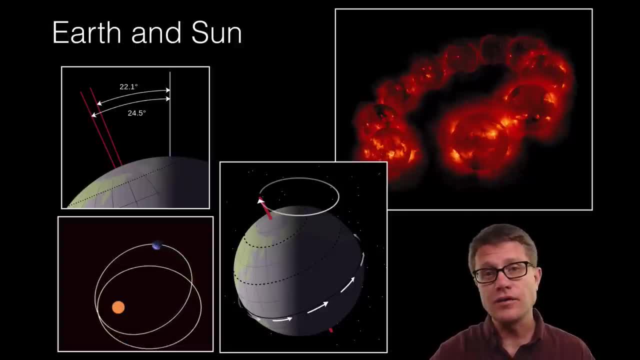 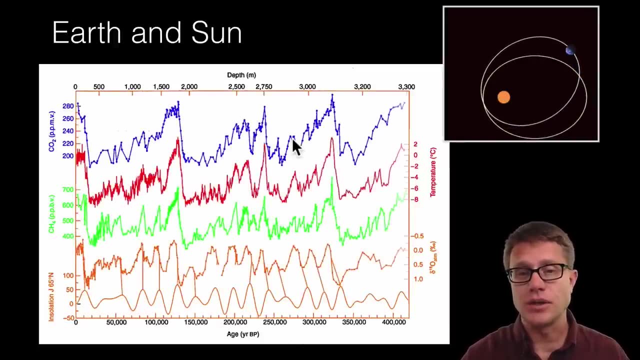 we have changes in the amount of energy that we are getting from the sun. So all of these changes correspond to changes in energy from the sun. So if we look at how these models match up with the data that we are collecting in ice cores, we can see the cycling of our 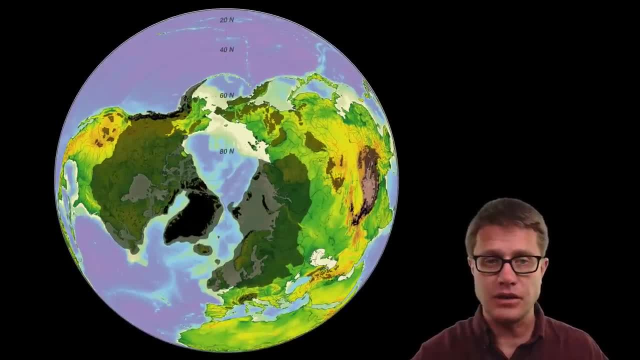 climate. over time We are going to have these ice ages And if we look down at the northern hemisphere, this is what it would be like during the worst ice age: That whole area that is gray would be covered in ice. That means most of Canada, Great Britain, all of Scandinavia. 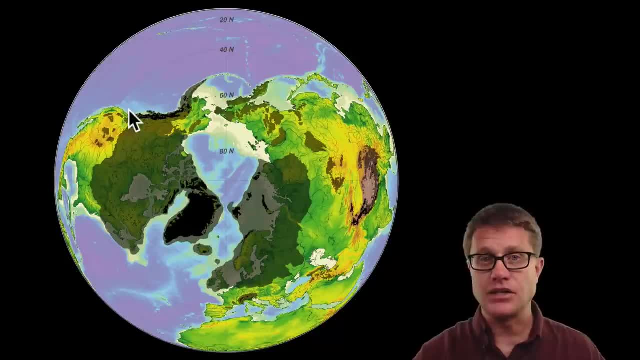 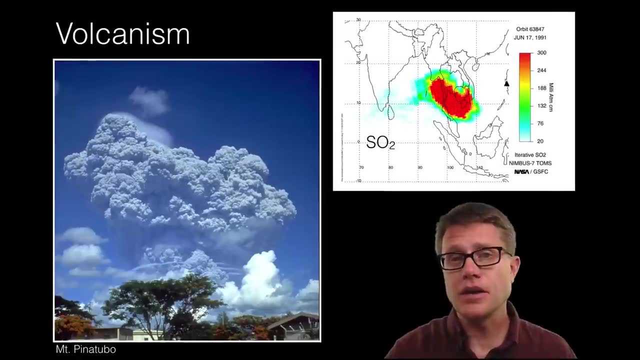 would be covered. It would move down into the US as well- Massive ice sheets, And then we would have times where there is not much ice at all, Just this dark area where Greenland is, and then along the coast right here. Another thing that can affect climate is going to be volcanoes, And so, for example, in 1991 in the Philippines. 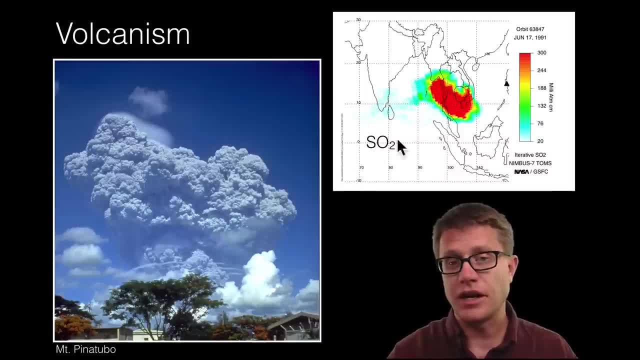 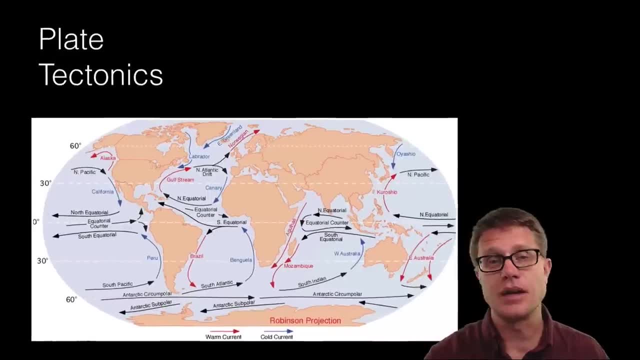 Mount Pinatubo exploded. That increases the amount of sulfur dioxide in the atmosphere and it cools the planet. So the planet cooled over the next three years just due to this one eruption And then we can have plate tectonics. that is affecting the amount of energy we 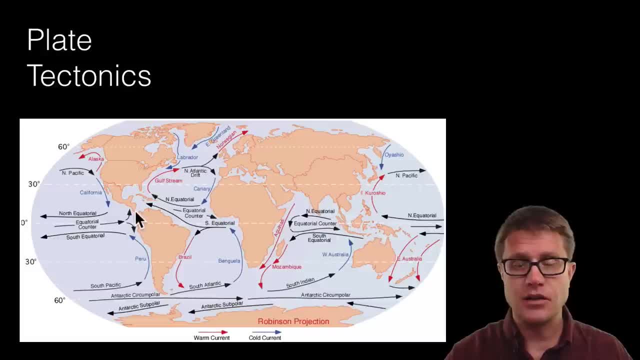 get as well. So a simple example: South America slid into North America and Panama was formed. What happened? there used to be a current that moved through here and that changed the whole current, And so that is going to affect the climate Where at the largest level- Pangaea- 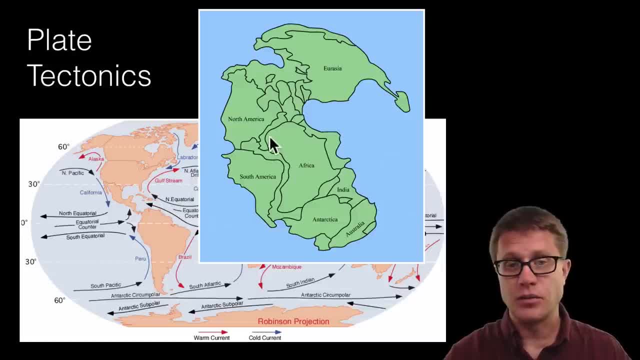 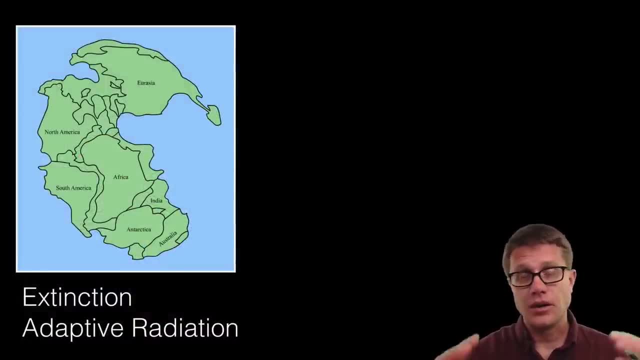 was all of the continents coming together. We have massive deserts forming in the middle And that is going to change species on our planet. It led to some of the worst mass extinctions on our planet, where a large percent of life actually went away. Now this changed eventually. 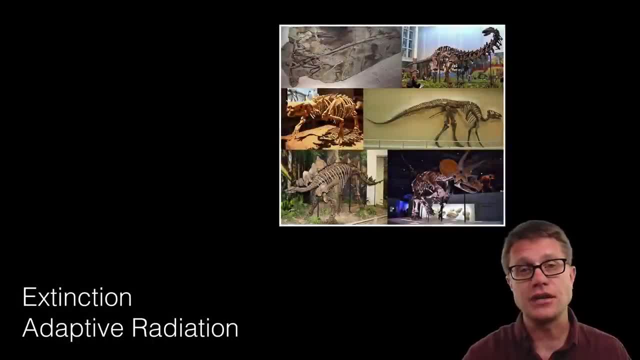 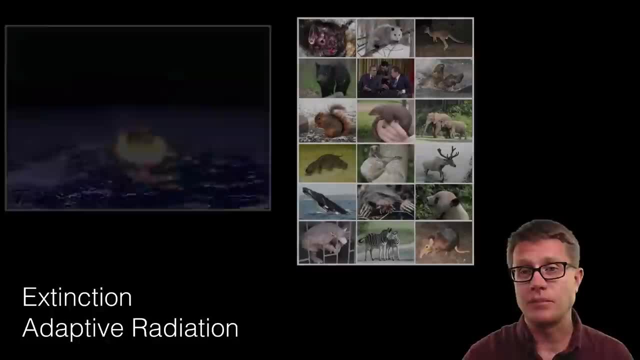 as they broke apart. We had an adaptive radiation and all these dinosaur species showed up. What happened to them? giant asteroid impact, mass extinction, and that led to adaptive radiation of the mammals, And some people are saying we are headed into a sixth mass extinction And so this is the 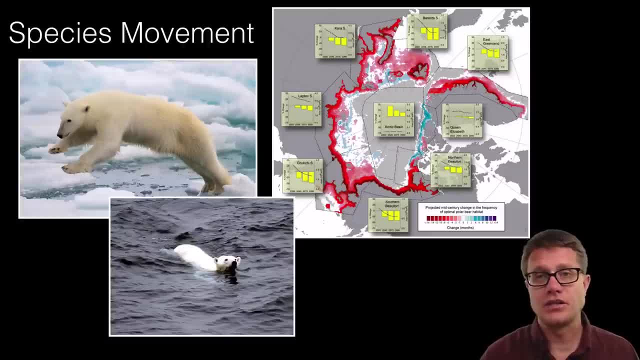 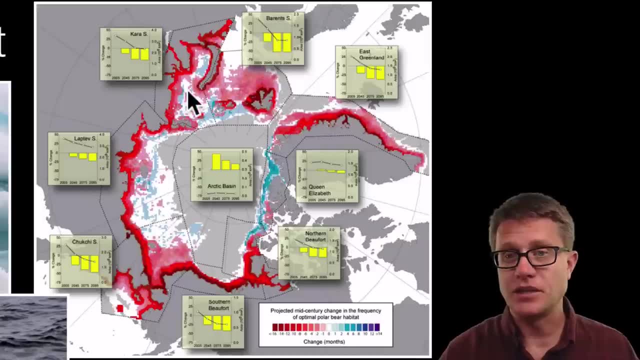 worst way that climate can affect species. Now, as the climate changes, animals can move, And so polar bears are going to be impacted. This is a distribution of prime polar bear habitat, And you can see it is being impacted all the way around the pole. Now, if polar 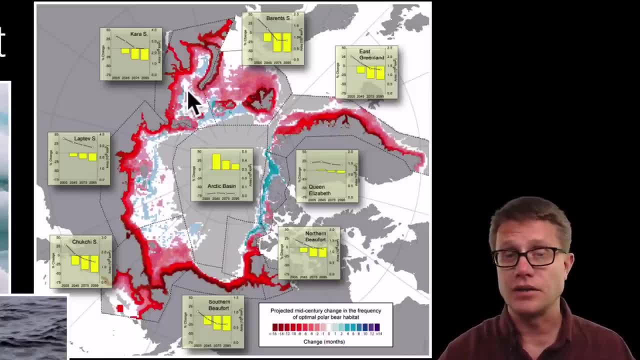 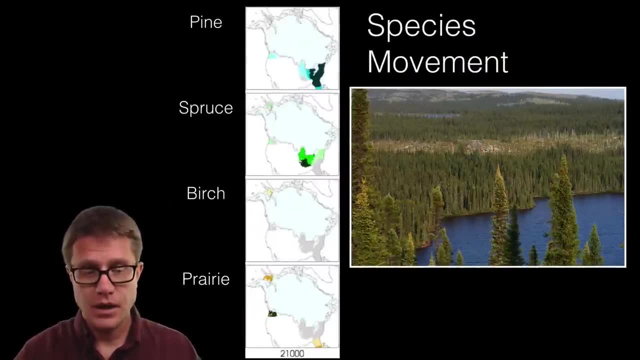 bears do not go extinct. what are they going to do? They are going to move into new areas and they are going to exploit new niches. Plants will do the same thing, And so, as the planet has gotten warmer and warmer and warmer, this is a distribution of prairie birch. 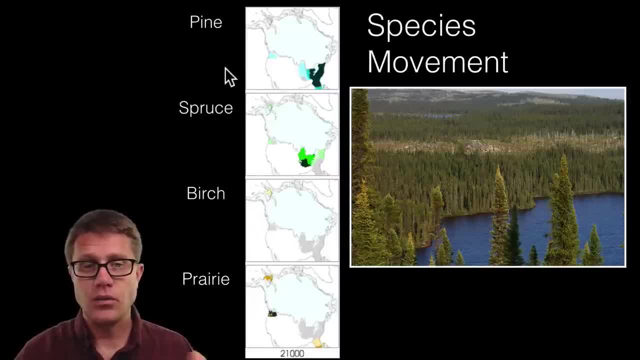 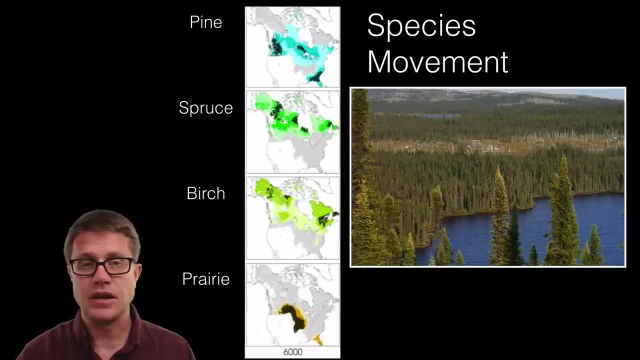 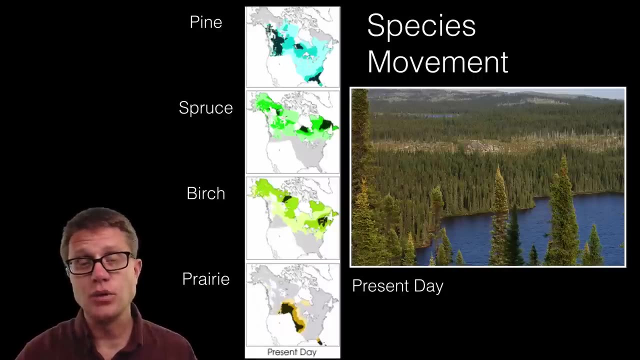 spruce and pine trees over the last 21,000 years And so watch what happens to their distribution. So now we are looking at 12,000 years ago And now 6,000 years ago And now present day distribution. So you can see that as the ice retreated, the plants moved into.